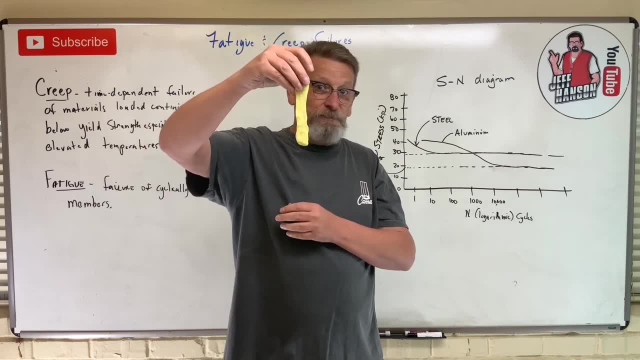 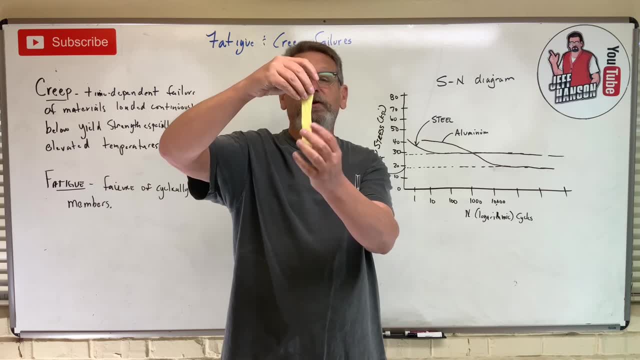 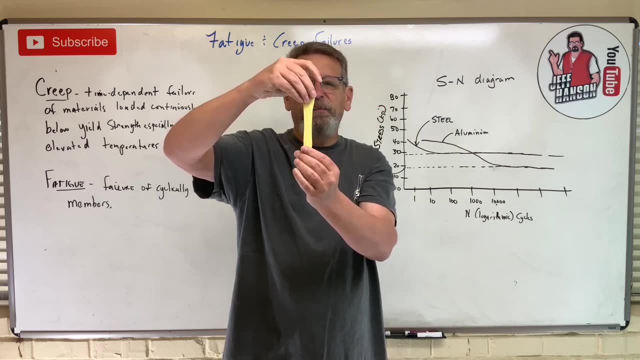 its own weight If I hold it here long enough. right, it's creeping. right now, As I hold this, it's elongating, It's getting longer. okay, I'm going to speed it up a little bit. pull on it. 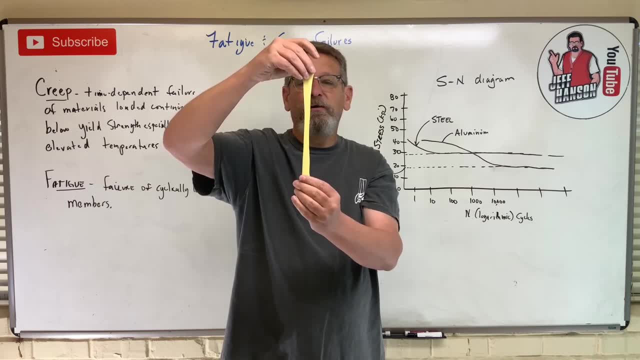 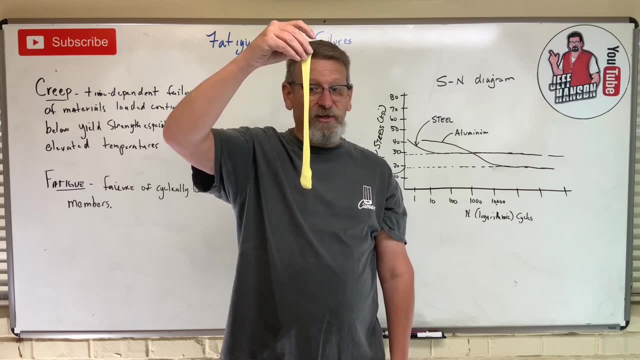 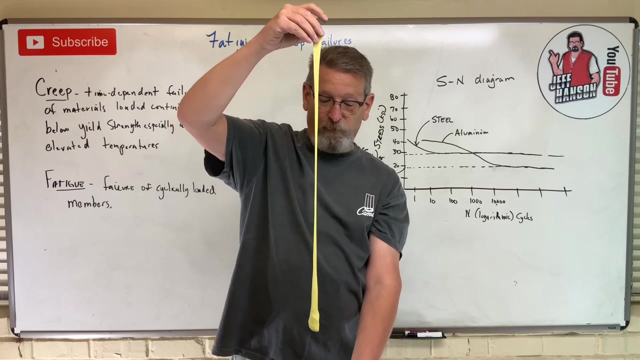 right Now, let's get a little bit longer. okay, It's still it has. now it's just under its own weight. It's starting to elongate, okay, And when it gets down to a certain point it'll elongate more and more and more. Now it's moving on its own without any other applied force. 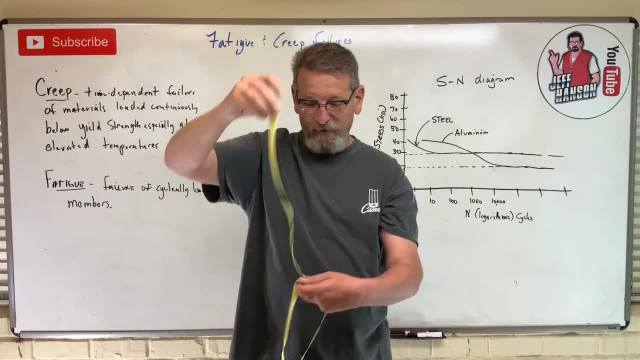 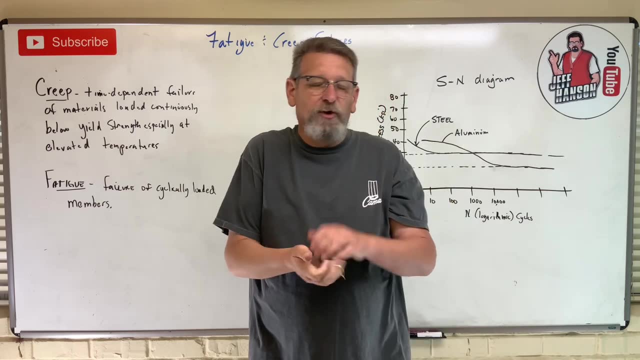 It's getting longer and longer. It eventually is going to fail, isn't it? Okay, that's creep, something that's just moving under its own weight from continuous load. Now, you don't make many things out of silly putty, okay, Thankfully. 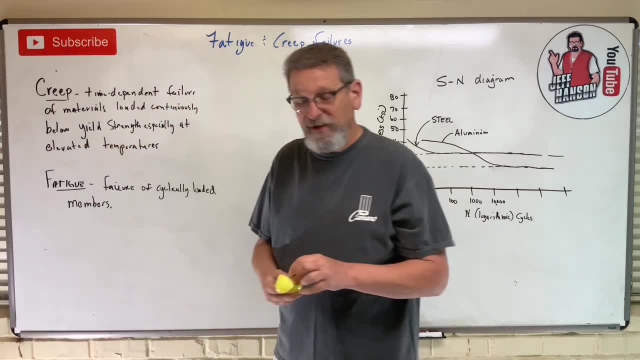 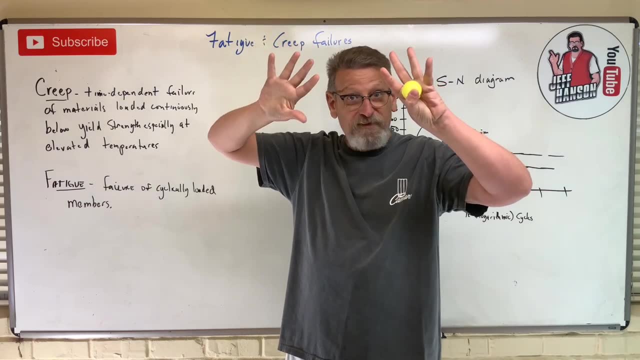 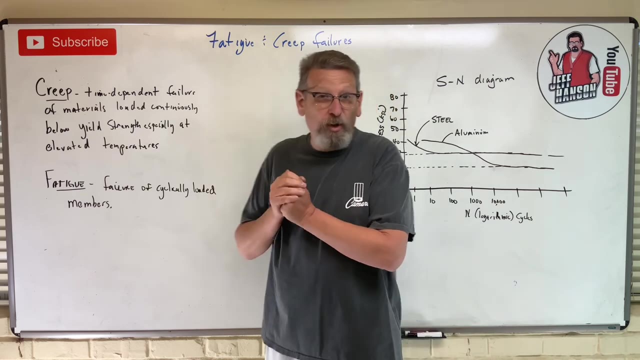 But we do see things like glass. Glass, as it's continuously held in one place, over time will start to sag. It's actually moving. It's like a liquid actually, But you can see that under things like especially like in boilers or things where things. you get an elevated temperature and it's under continuous load, it will eventually grow enough that it will cause a failure- a leak or a crack or something like that could happen. So that's creep, a time-dependent property of materials that allow it to fail over long. 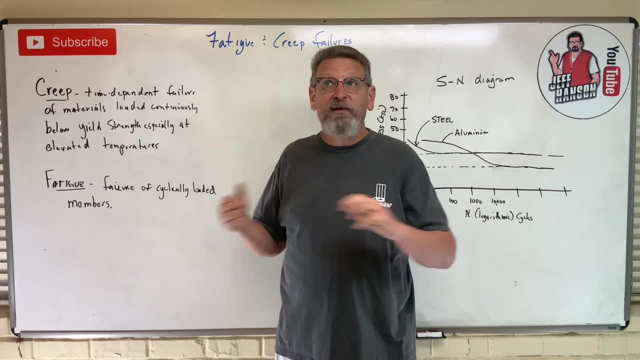 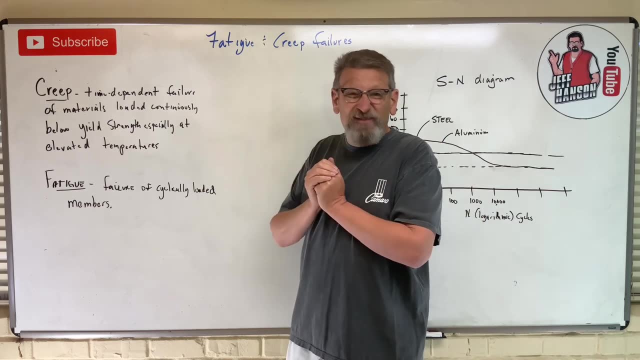 long periods of time. Now it's a long period of time Like a boiler might fail after like 100,000 hours of heat cycles, heat loads, And so you know that's a long long time, But 20,, 30 years maybe we can have a failure from creep. The second one is that you may be more. 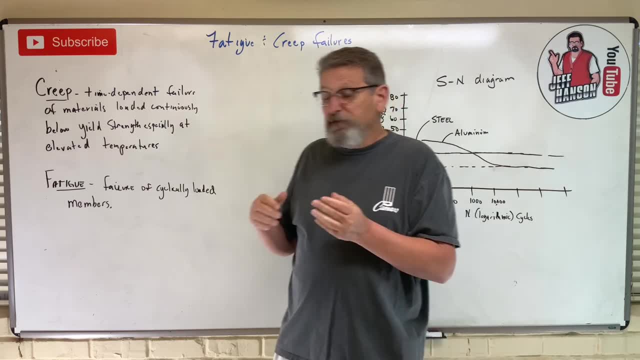 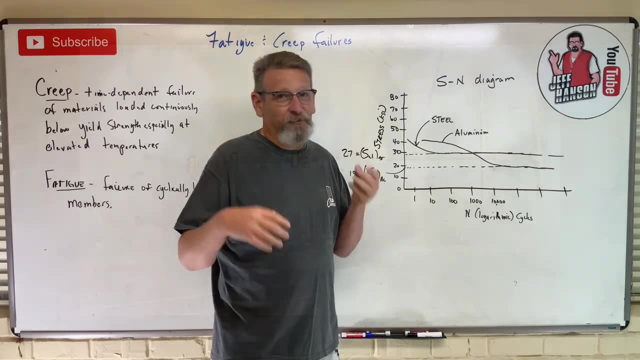 familiar with is fatigue. okay, So fatigue is the cyclical loading of members. One of the things that I see here all the time, especially in West Texas when the wind blows, is this: okay, Notice how the traffic lights out here when the wind starts blowing. 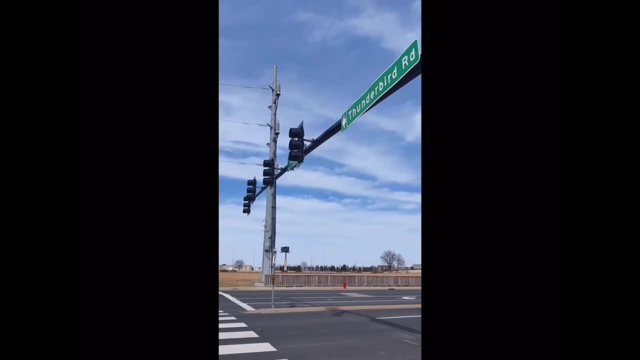 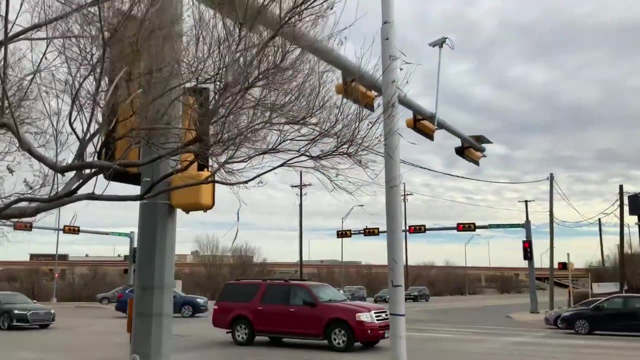 the traffic lights start oscillating And where those traffic lights are connected to the ground, those bolts are going under a load like tension compression, tension compression, tension compression, as that beam cycles up and down, So on the downward it's in tension On the 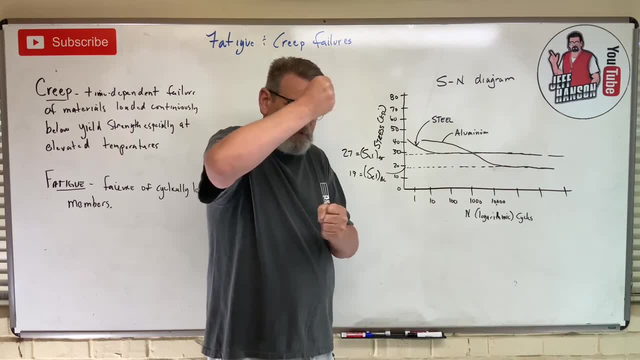 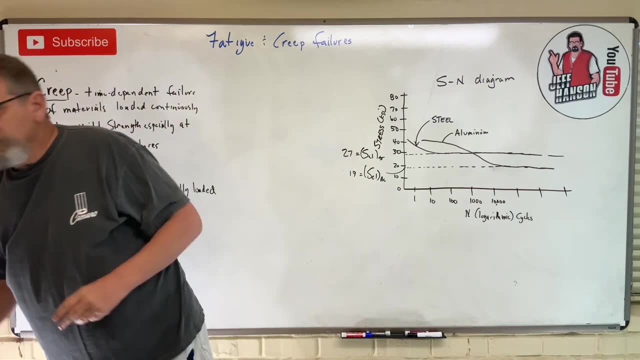 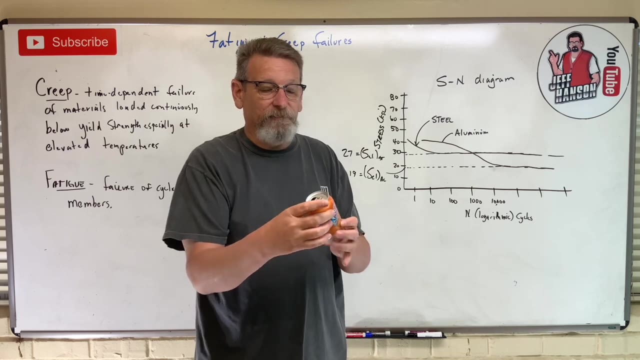 upward, it's in compression, So that loaded member is just being Compressed and stretched, compressed and stretched, compressed and stretched. Now we know what happens on these things, Some things that we might see. okay, Number one: here's just an old pop can, here, right, A little soda can, And it's got the old pop top on it. 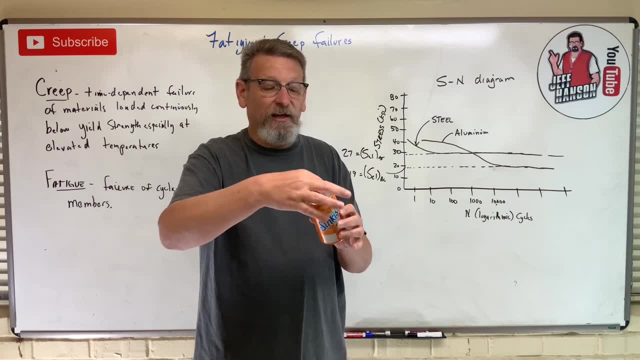 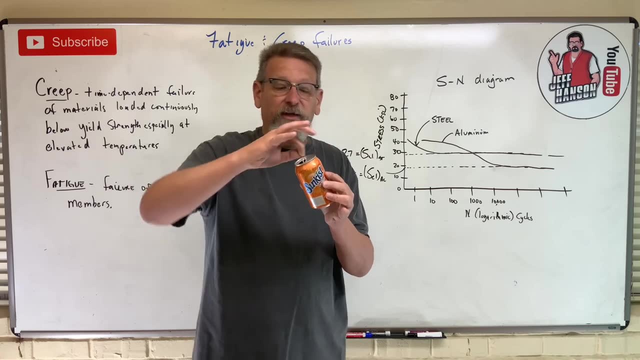 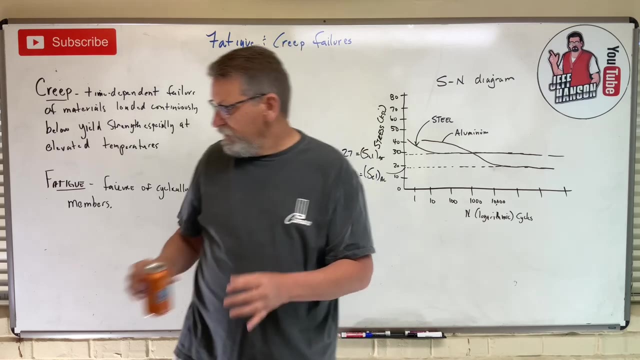 okay, Now, fatigue failure. How many times can I load this and unload it, and load it, and unload it, and load it, and unload it, and load it, and unload it before I have a failure? okay, Now, that's something we're very, very familiar with, Things that we don't like. 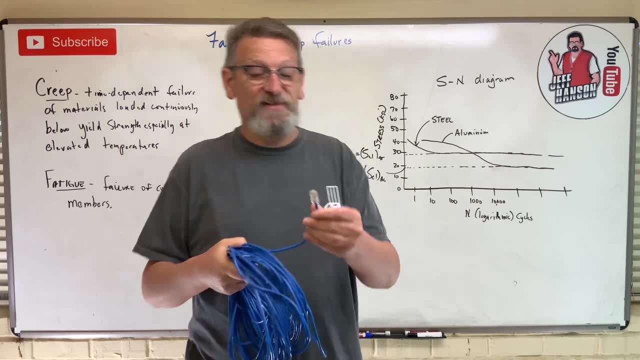 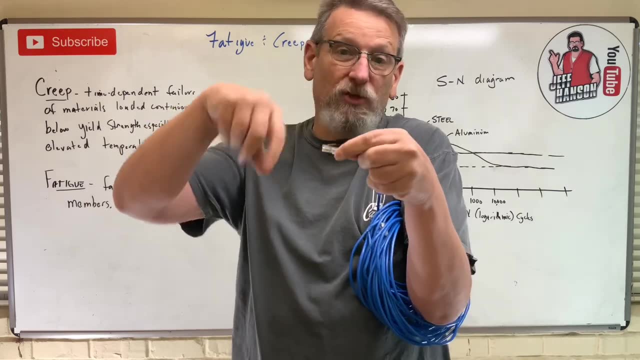 Some of my people told me that y'all wouldn't know what this is. but I think you all know what this is, right. This is a little clip on the end of your ethernet cable here, right? How many of you have one of these where you hook this on the carpet and you've pulled that back and you pull? 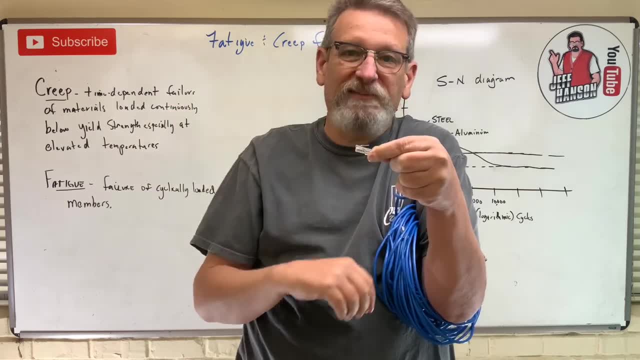 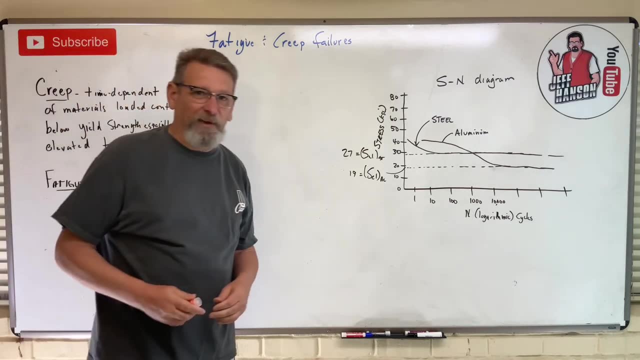 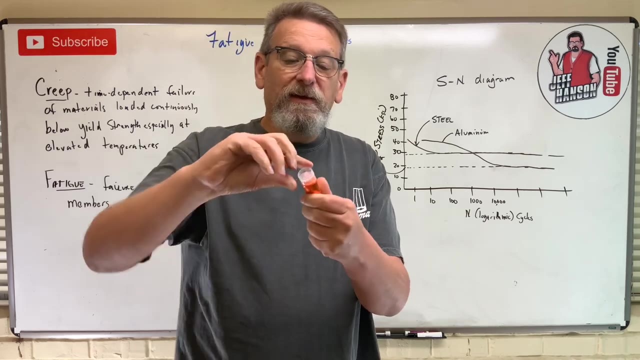 it back and a couple of times and that little plastic tab there breaks off. That's a little fatigue loading, right. But then we have other plastic materials, like this little cream bottle here. It has what's called a living hinge on it, okay, And it has a little plastic connected hinge. 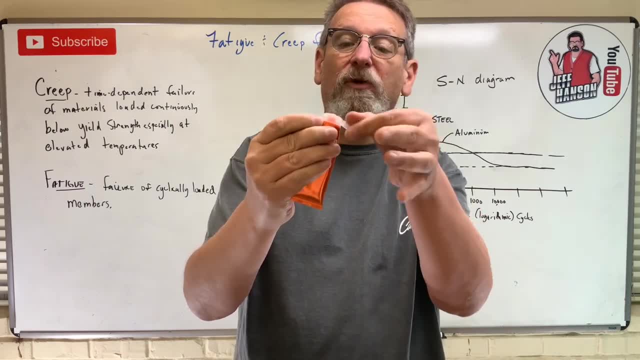 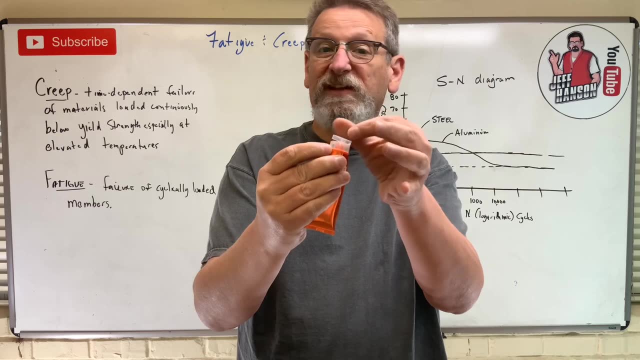 on it right here, but I can fold that back, forth, back forth. I can fold that for hundreds and thousands of cycles and it will not fail. It's designed to do that. It's called a living hinge. It might fail after a long, long time. 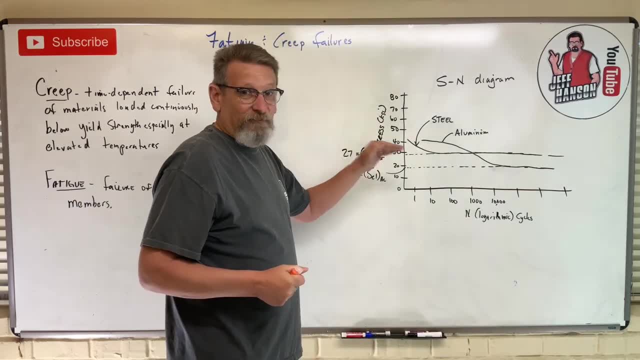 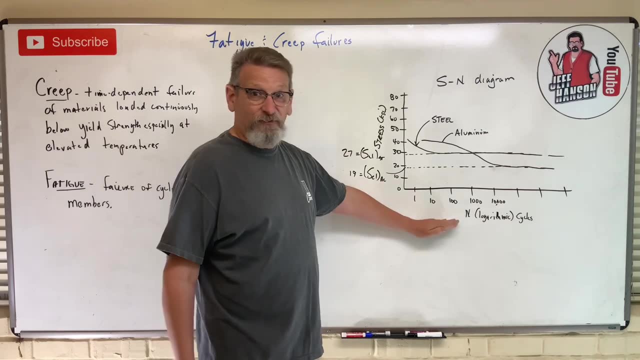 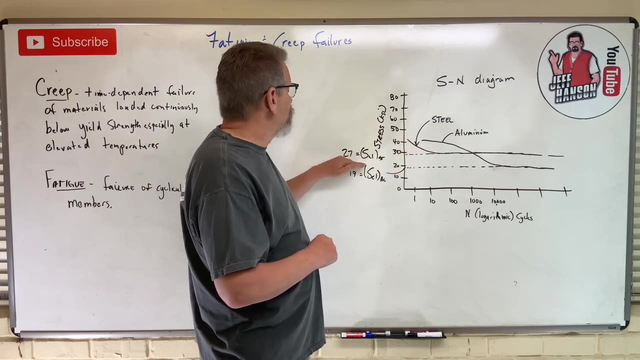 but what we have here is something called an S-N diagram for materials. okay, And what is the S-N diagram? S stands for stress, N stands for number of cycles. So steel, if I stress it, below 40, right, If anything below 27,, even if I load it and unload it, an infinite number of cycles. 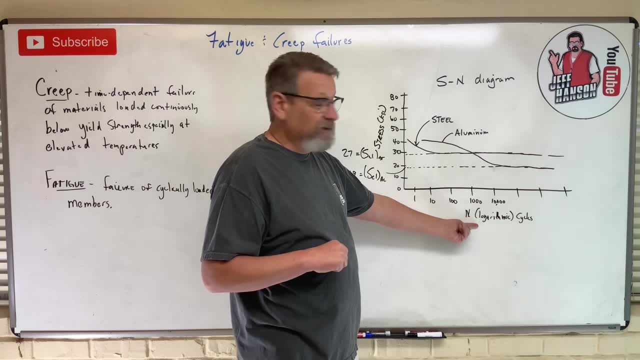 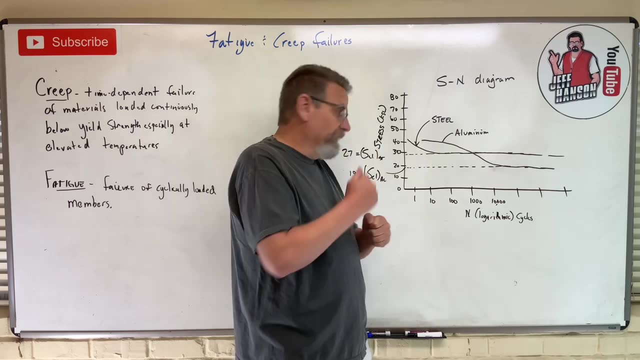 okay, Now this side, the column down here, the axis down here for cycles is logarithmic. okay, This is the number of times something is loaded and unloaded, loaded and unloaded, And what this line here shows is that steel when it gets down to 27.